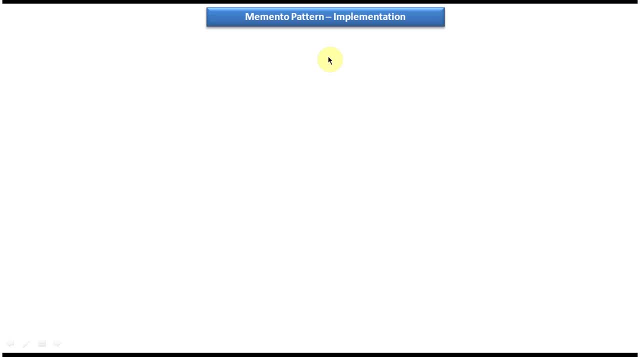 Now we will see the scenario of Momondo Design Pattern. So I buy a 42 inch LED TV, which is 60,000 rupees and it won't support USB. So I buy this LED TV and I placed it in the hall. So after some point of time I am thinking: ok, let me buy a 46 inch LED TV. 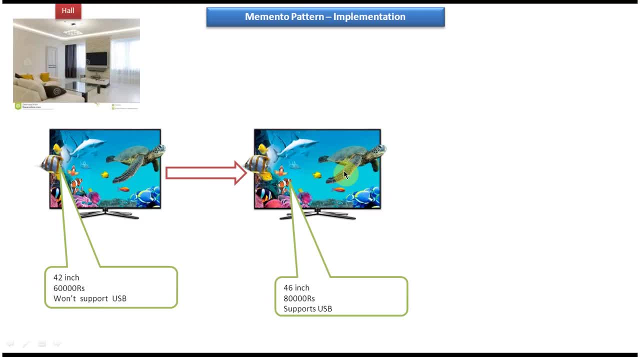 So I buy a 46 inch LED TV, which is 80,000 rupees, And this 46 inch LED TV supports USB. So what I have to do is I have to place this one in the hall. So, already in the hall, 42 inch TV is there. So what I have to do is: 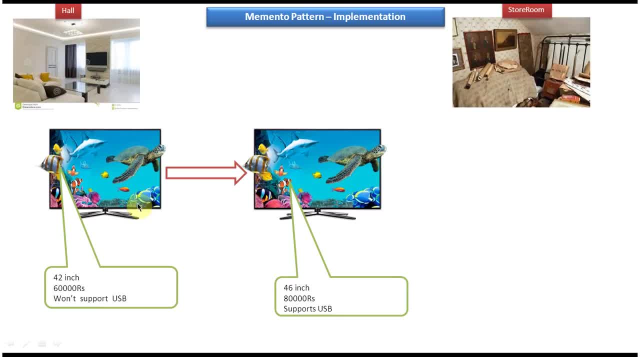 I have to put this 42 inch LED TV in the store room And place this 46 inch LED TV in the hall. After some point of time I am thinking: ok, let me buy a 50 inch LED TV, Which cost 1 lakh rupees and it supports USB. 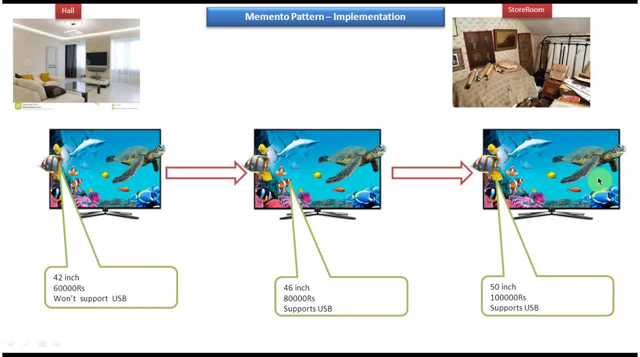 So I buy this 50 inch LED TV, Then what I have to do is I have to place it in the hall. But in the hall now, 46 inch LED TV is there. So what I have to do is I have to take 46 inch LED TV from the hall. 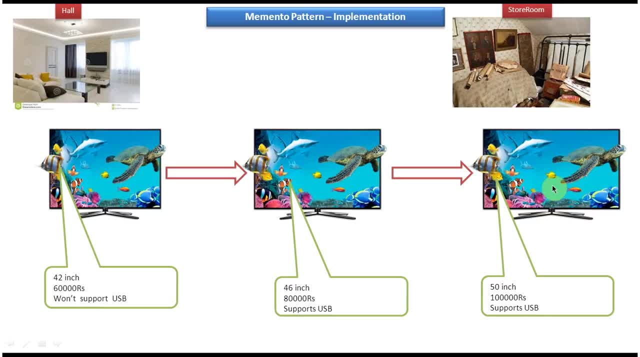 And put it in the store room and place this 50 inch LED TV in the hall. So in the hall, what is there is 50 inch LED TV. So after some point of time I am thinking, ok, let me use 42 inch LED TV. 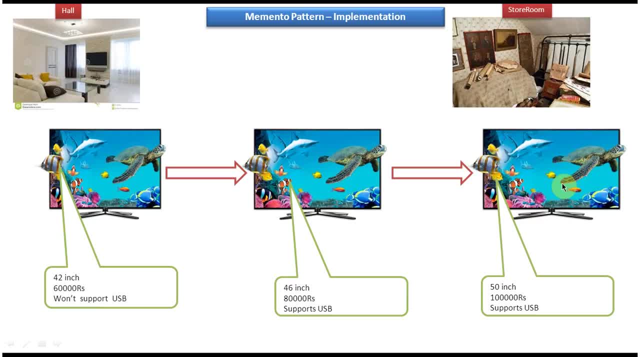 The clarity of 50 inch LED TV is not good, So I have to basically restore or roll back. So what I have to do is I have to put this 50 inch LED TV in the store room And from store room I have to take 42 inch LED TV. 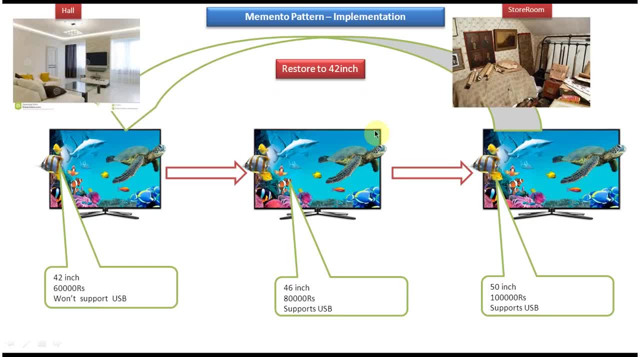 And place it in the hall. So basically, what I am doing is I am roll back to the previous state. Ok, this is the best example of Momento design pattern. So this kind of restore or roll back scenario, we can use Momento design pattern. 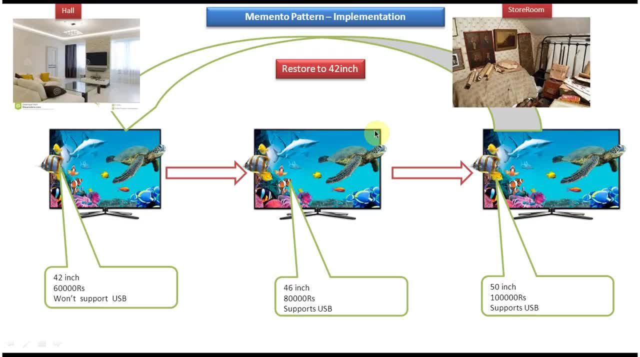 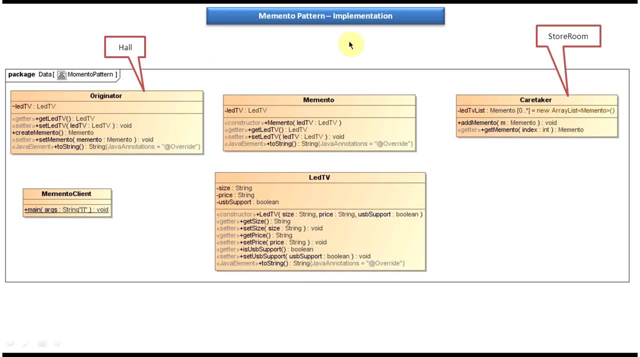 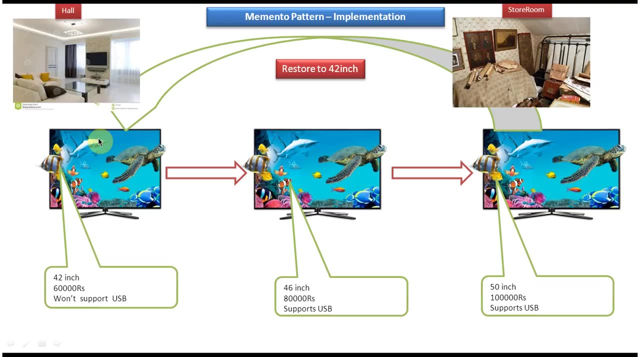 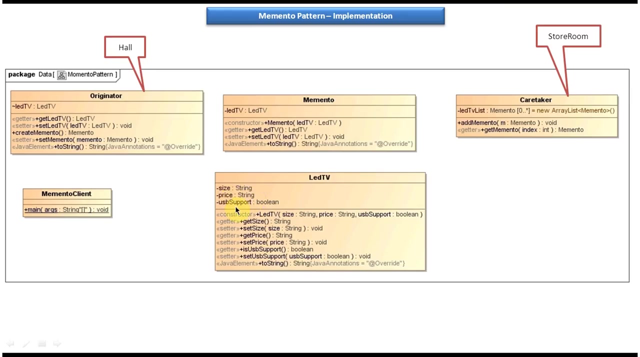 Ok, now we will see the class diagram of this scenario. Ok, this is the class diagram of the scenario which we have just seen. So here you can see LED TV class, Which represents LED TV. It has three attributes: Size, price and USB support. 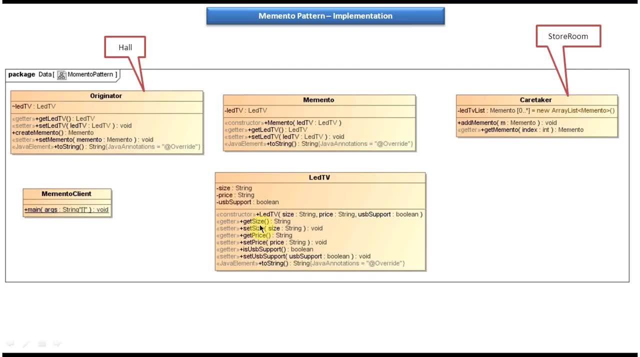 And it has getter and setter method for size, price and USB support. Suppose. if you want to create LED TV object, You have to just call this constructor. by passing Size, price and USB support And left side, you can see originator. 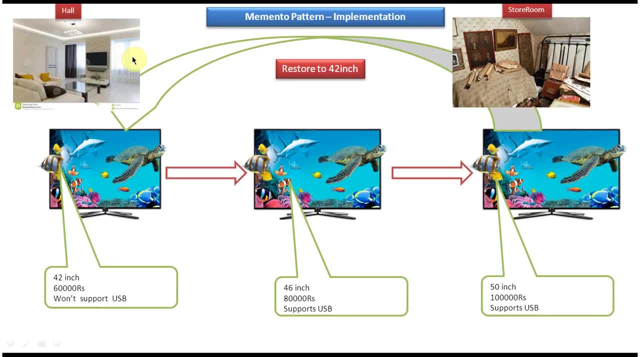 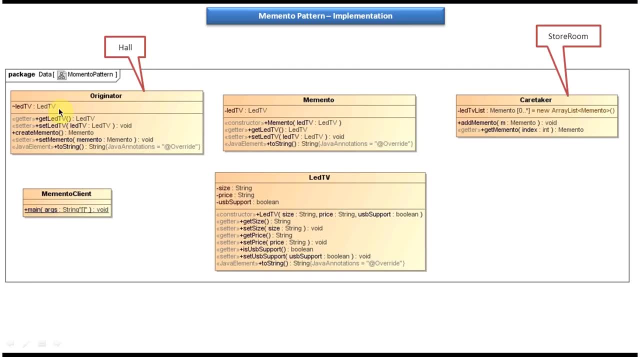 Which is nothing but hall Which we have seen here. So this hall has LED TV object And getter and setter method for LED TV And the originator has createMomento method. So what this method will do is it will create the Momento object. 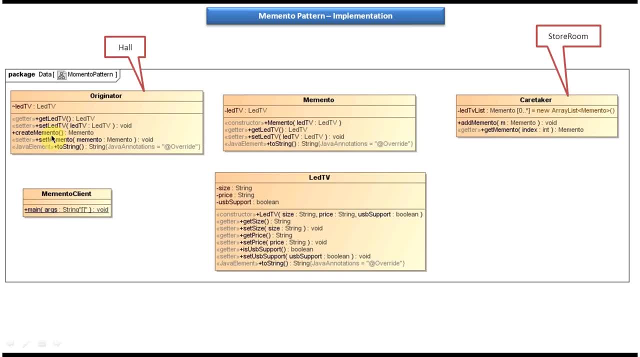 And it will set originator internal state to the Momento And basically this method is used to take the current snapshot of originator and put it in the Momento And it has another method called setMomento And parameter should be Momento object. 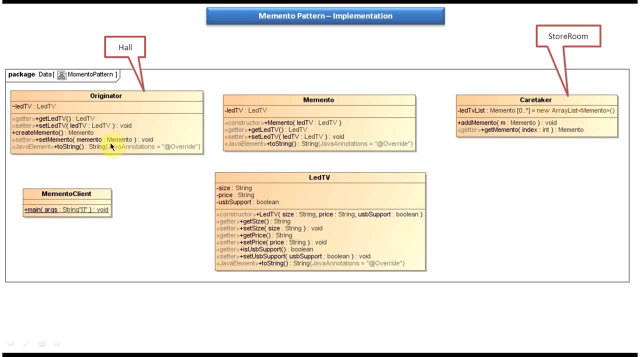 So what this method is doing is It will take state from the Momento object and set it to the originator. Basically, this method is used to restore or rollback And Momento object. So it has LED TV which hold the internal state of originator. 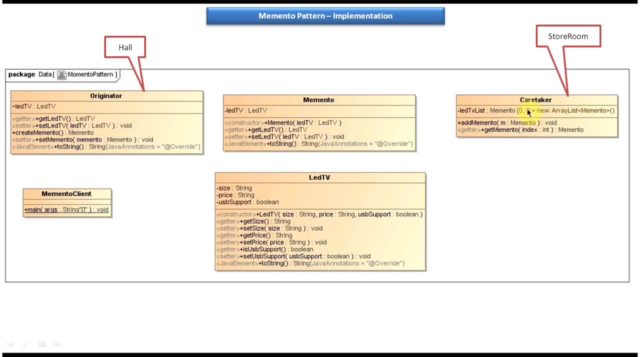 And right side you can see caretaker, Which is nothing but storeroom, which we have seen. And so what is the use of caretaker? is It will maintain the Momento object. So here it maintains the LED TV as a ArrayList. 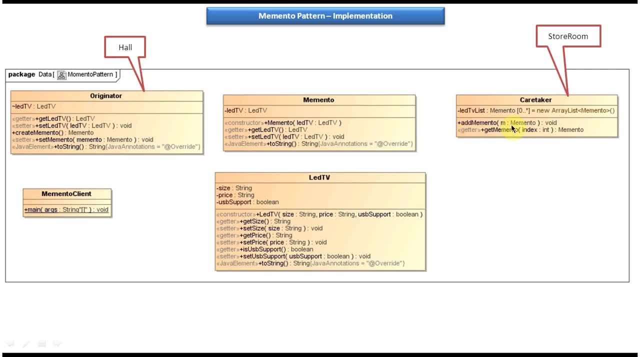 And it has method to add the Momento object to this particular ArrayList And it has getMomento method. Here you have to pass the index. So based on the index value It will give the particular Momento object Okay, Suppose you want to restore or rollback. 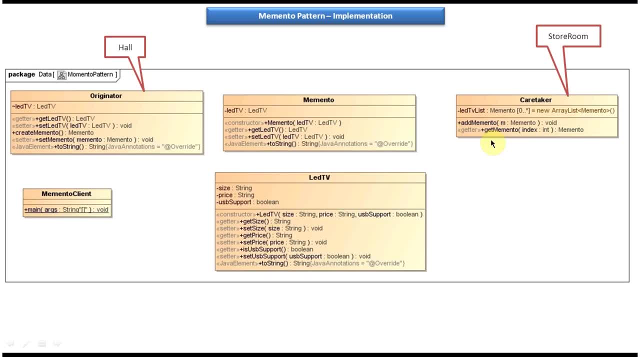 Then you can get the old Momento object from the caretaker by calling this getMomento method. Okay, So basically this is a class diagram. We will see the code in Eclipse. I will open the Eclipse and show you. Okay, I have opened Eclipse. 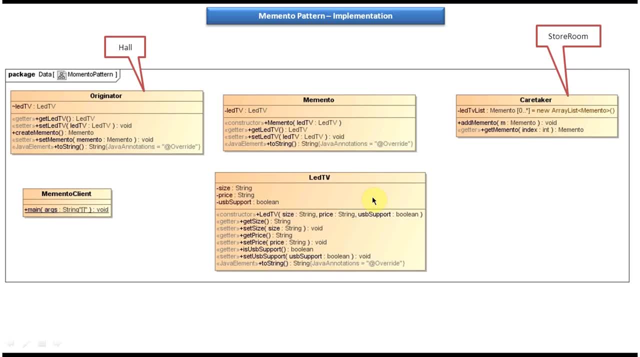 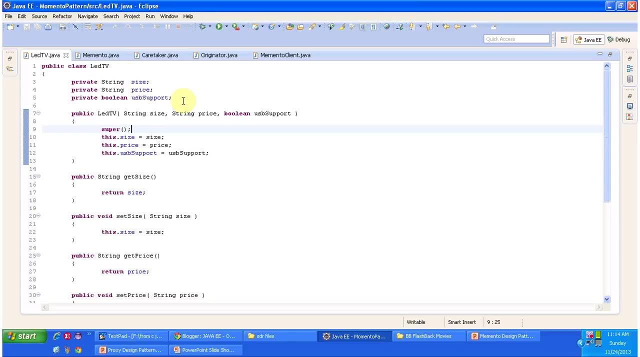 Now we will see the code, So in the down you can see LED TV class. So I opened LEDTVjava And it has three attributes: Size, price and USB support, And getter and setter method for size, price and USB support. 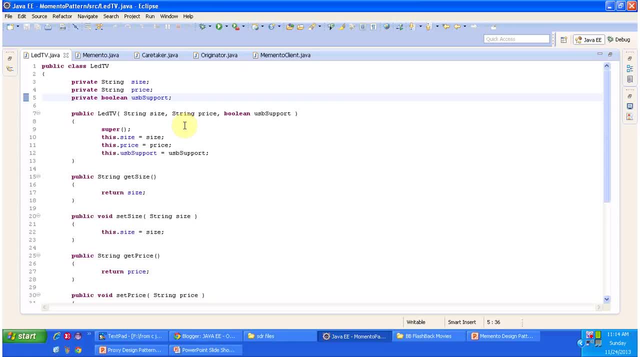 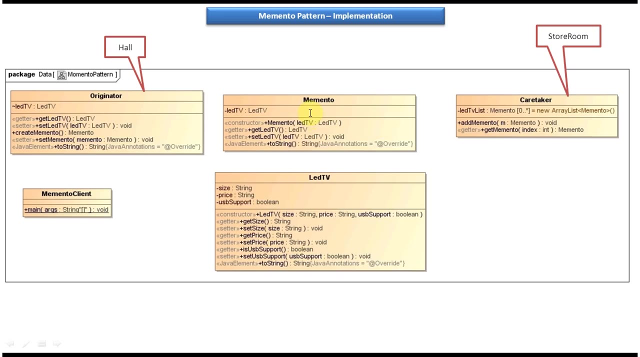 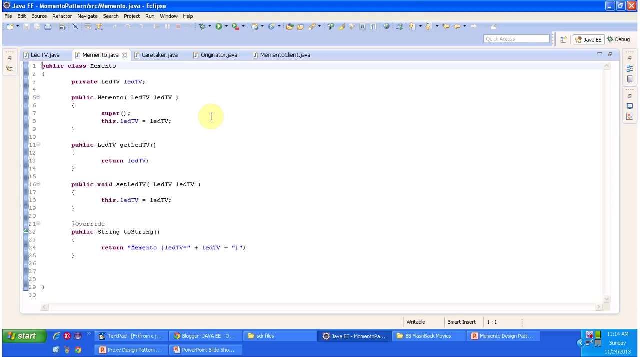 And it has LED TV constructor. Suppose, if you want to create LED TV object, Then you have to pass size, price and USB support to this constructor. Okay, And next class is Momento class. So I will open Momento class. So this Momento object is used to store the internal state of originator. 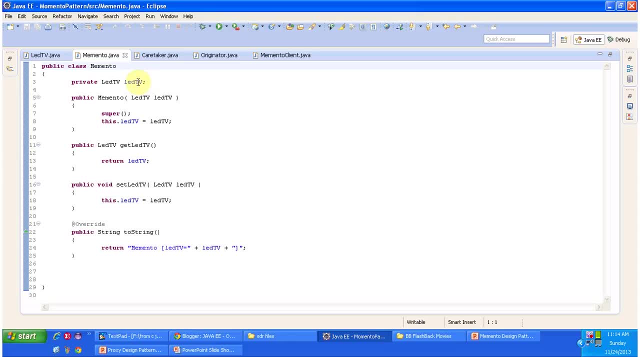 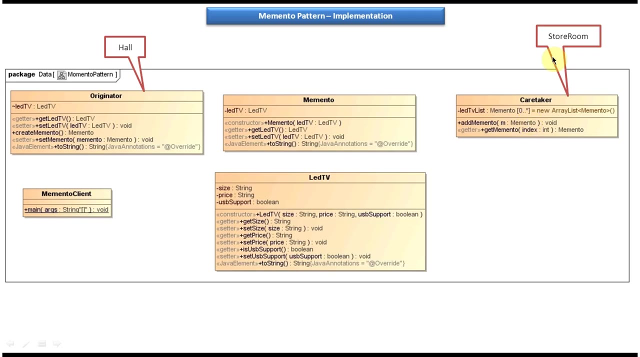 So the originator has LED TV as internal state, So it has LED TV here And setter and getter method for LED TV attribute And right side you can see caretaker which is nothing but store room Which is used to store the LED TVs, old LED TVs. 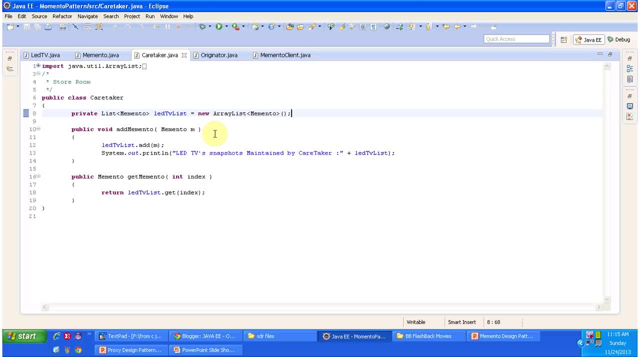 So I open caretakerjava And this caretaker is used to maintain the Momento objects And it has method to add the Momento in the LED TV list And suppose if you want to get old Momento object You have to just call this getMomento method by passing the index. 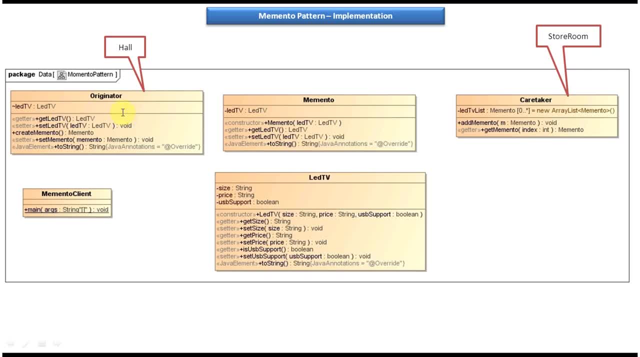 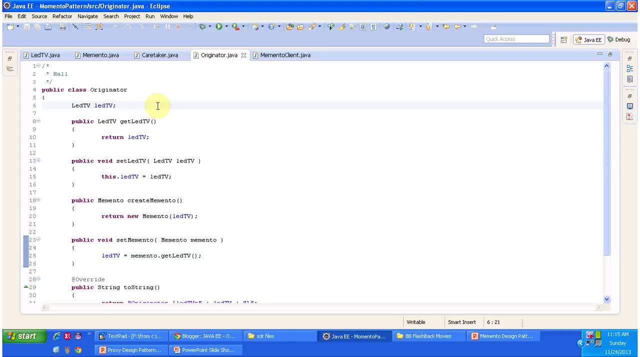 And next class is originator. So originator is nothing but a hall which has LED TV or LED TV in it And here you can see LED TV object And getter and setter method for LED TV object And it has createMomento method. 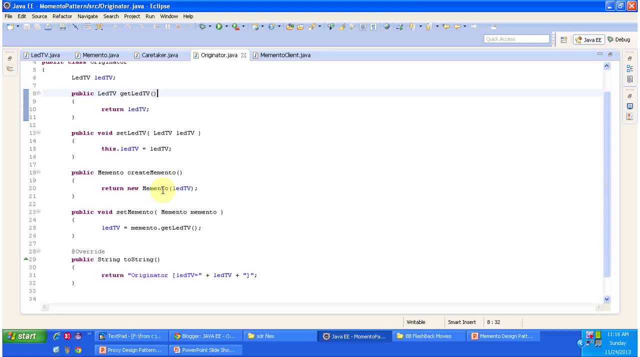 So what this method will do is It will create the new Momento object And set the originator internal state to the Momento object, And it has setMomento method. You have to pass the Momento object, So this method is used. 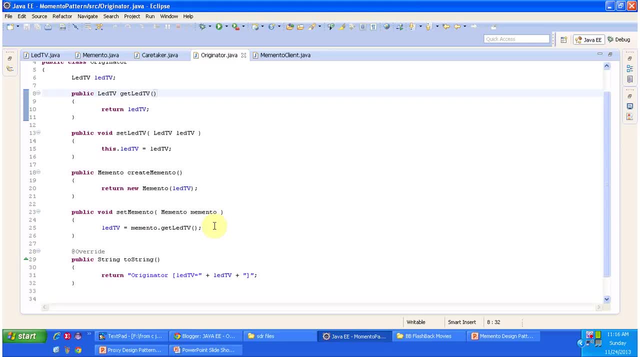 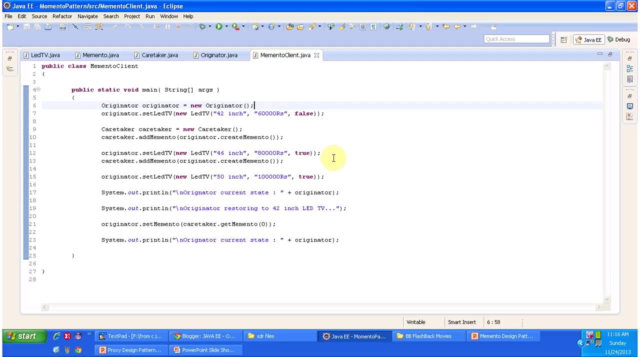 So this method is used for restore or rollback. So you have to pass the Momento object From the Momento object. it will get the internal state And assign to the originator internal state And next class is Momento client. So this is used to explain this Momento design pattern. 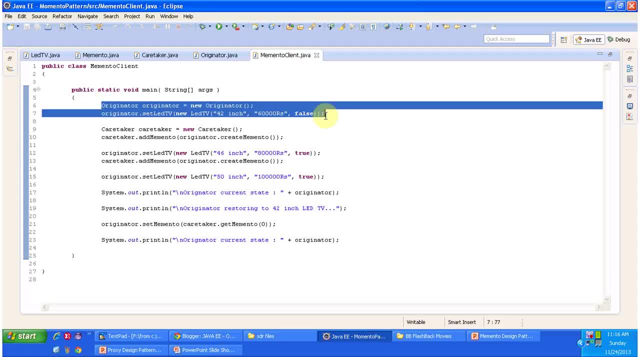 So initially originator has 42 inch LED TV. So originator is nothing but a hall Which has LED TV, And later I buy a 46 inch LED TV, So I have to move 42 inch LED TV to the storeroom. 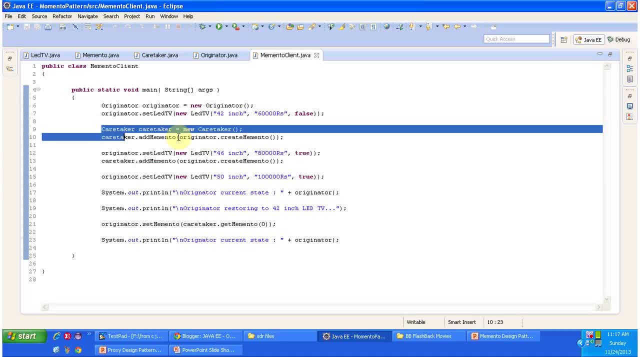 So in this case caretaker is a storeroom, So I am creating the Momento object And adding to the caretaker. So like that, later I buy a 50 inch LED TV, So I have to put 46 inch LED TV in the storeroom. 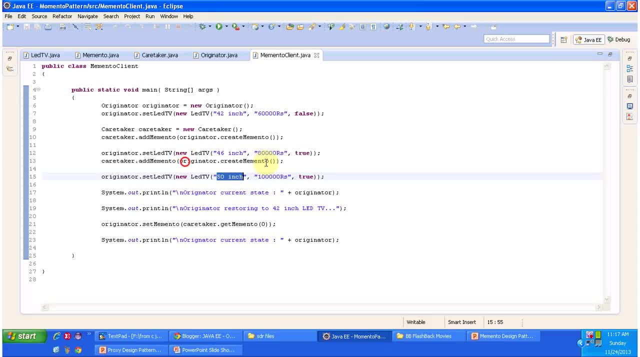 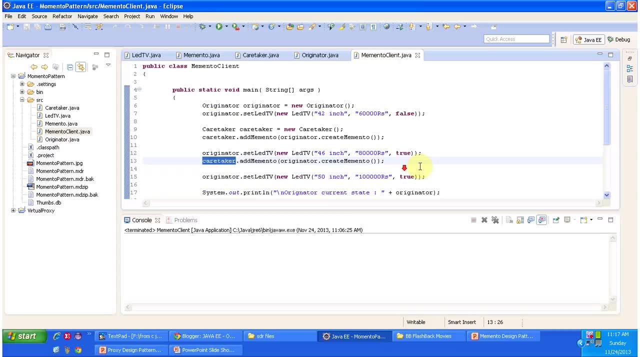 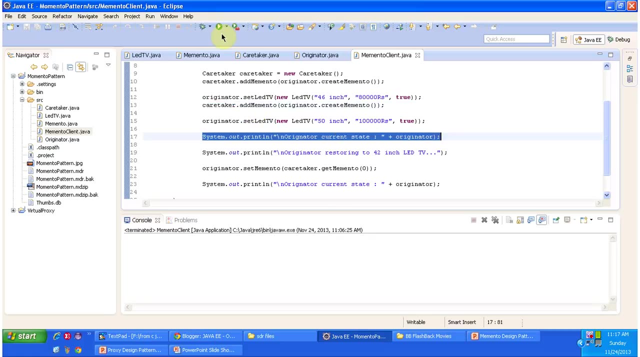 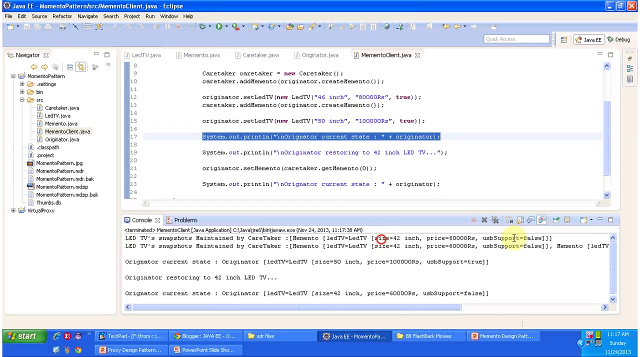 So I am creating the Momento object And put it in the caretaker. So now the current state of originator is 50 inch LED TV, So I will just run this one So you can see caretaker. initially it has 42 inch. 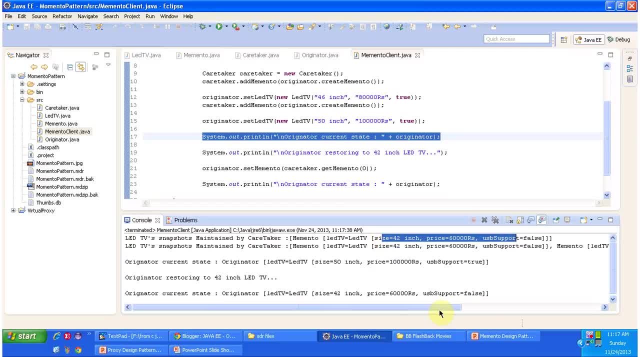 After that I am adding 46 inch LED TV, So you can see caretaker has 2 LED TV in it as a list And current originator state is 50 inch LED TV And after some point of time I am deciding to restore it to the 42 inch.